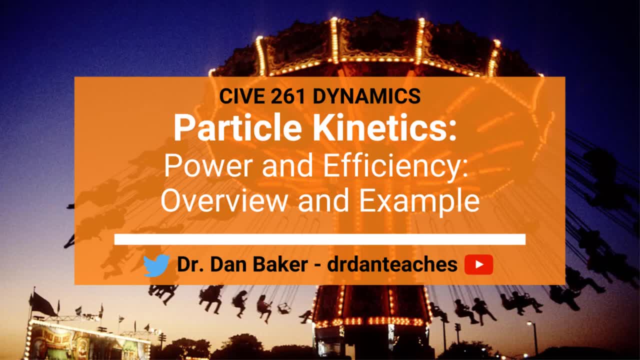 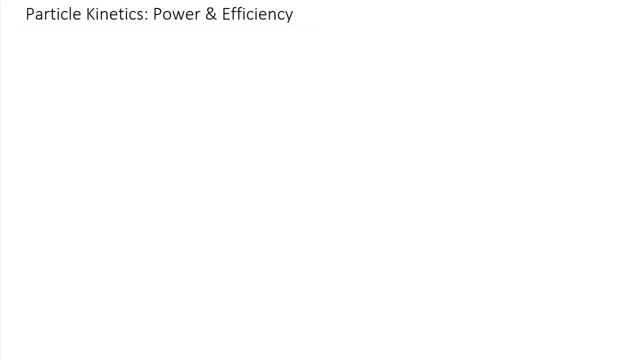 Hello, students of Dynamics. this is Dr Dan Baker and today's video we're going to take a look at particle kinetics, specifically power and efficiency. Now we don't spend a lot of time on power and efficiency, it's actually just kind of one section, but it is worth mentioning as 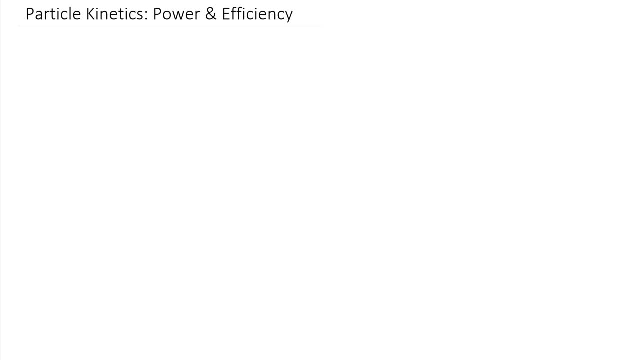 they're kind of an alternative to using a work and energy based approach. It's actually related directly to work, So let's go ahead and define power. Okay, so power we use. the variable p is defined as the time rate of change. 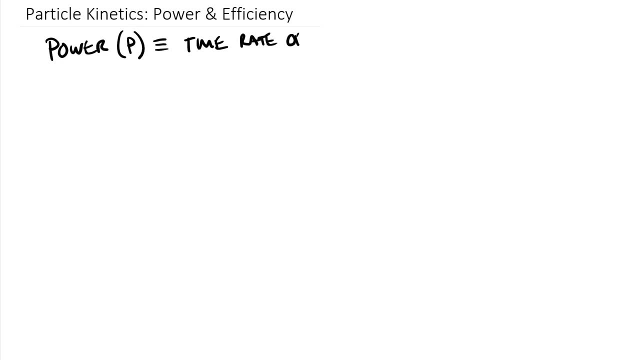 of work. Okay, so, given those words, probably not a surprise that p is equal to dw: dt- time rate of change of work. Now, while we could definitely compute power in this way, it's not always accessible to have work basically a time function of work, right? 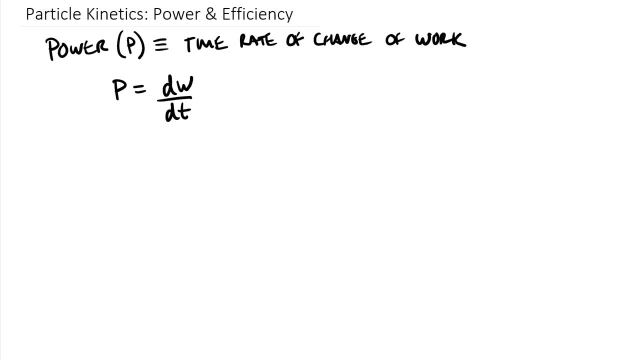 that recorded work over time isn't the easiest number to compute, And so what we can do is we can do a little substitution, And the substitution we're going to do is related to this work term. So if I make a substitution, remember that work is a dot product of force and distance. So we can. 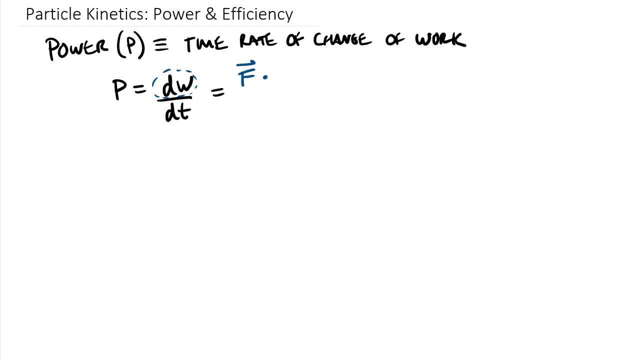 write here that work is equal to force dot, dr. Now, the reason it's dr instead of just r is because this is dw, right. it's an infinitesimally short amount of time over which we're doing work, And so this is going to be dt, right, so dt in the bottom, And then we can make one more. 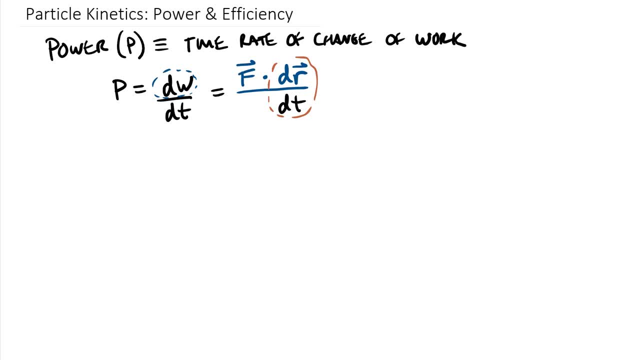 substitution here and that's related to dr dt. And of course we know that dr dt, the time rate of change of the of the position is the velocity. So the form of power that is a little bit easier to use is our force, f. when a dot that with our velocity, v. Okay, so if you find your instantaneous, 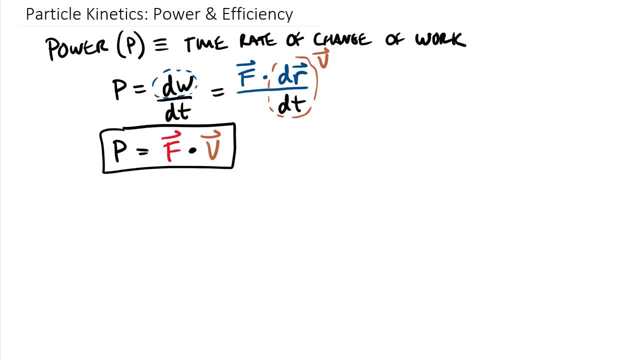 force and your instantaneous velocity. it's going to be the velocity v And then we're going to write velocity. if you dot those two, you end up with an instantaneous scalar value of the power at that moment. So if we think about the units for power in SI units, power is often expressed in joules. 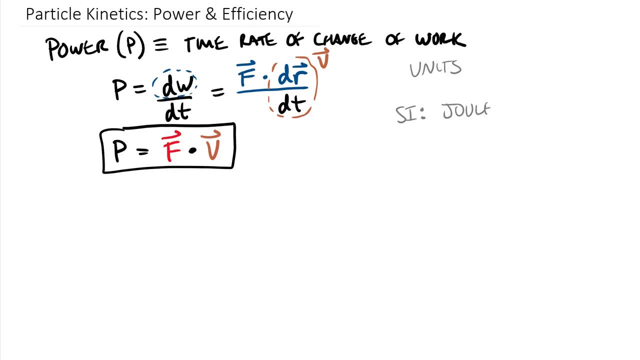 per second right, which joules is our work term, which is equal to a newton meter. And this joules per second is also equal to a watt. Okay, so a watt is a joules per second. And then in US customer units- not quite as tidy of units here- certainly we can express: 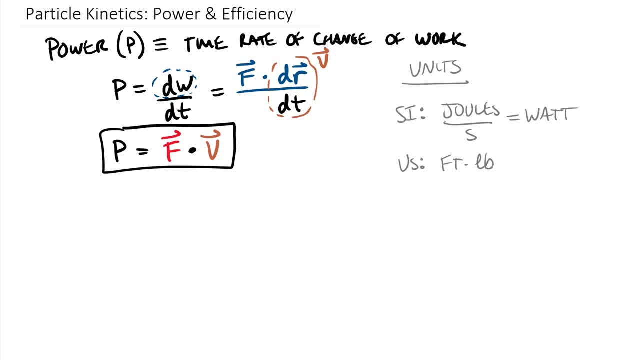 it in foot pounds per second. Okay, so that would be our work per time. Or we can also use horsepower. Okay, Now notice, I'm putting or, as opposed to an equals, because there is a conversion here, and that is that one horsepower HP is equal to 550 foot pounds per second. 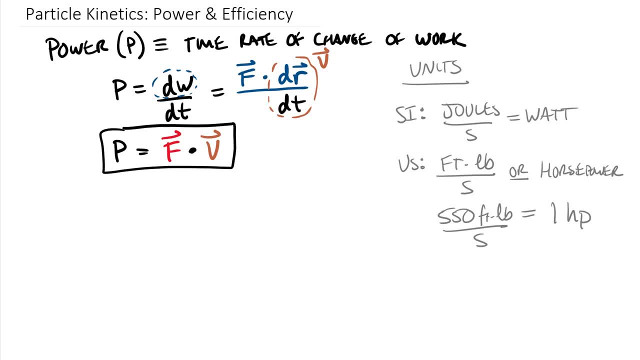 Okay, so you do that substitution just like you would. you know, 12 inches to a foot right. It's just a, It's just a substitution we can do for the units. So that's power. Next, looking at efficiency, 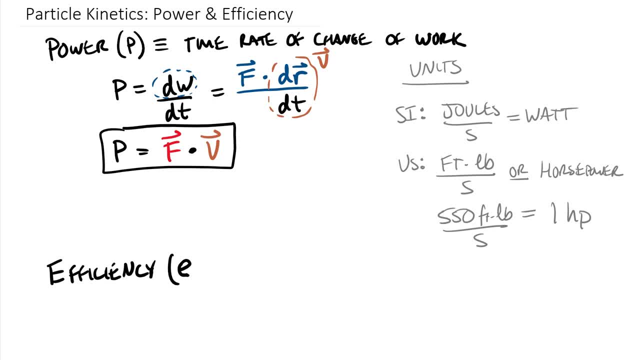 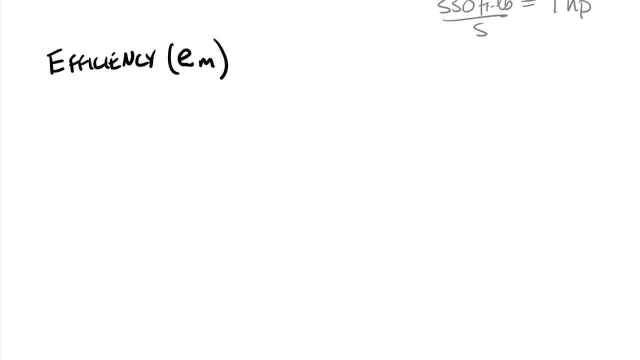 And efficiency. we can use small letter, e sub m. The m comes in because it's mechanical efficiency. There are other types of efficiency, So e sub m. Okay, Okay, Okay, Okay, Okay. Defined as the ratio of work done by a machine to the work done on a machine. 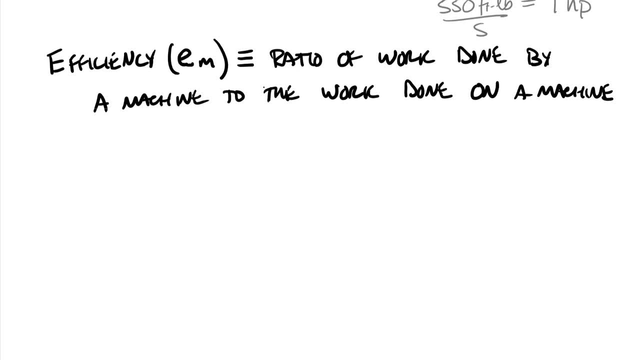 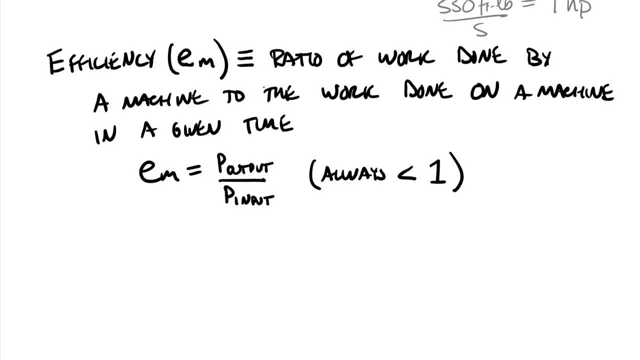 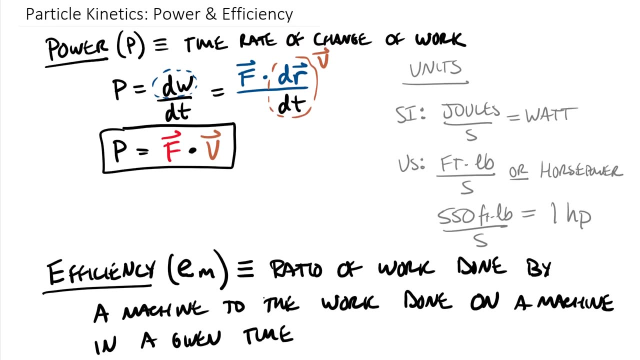 less than one. if you come to the system, you end up with more power coming out than power going in. you're either going to be a billionaire or you made a math error. okay, so that is the principles of efficiency and also power. so to demonstrate how we can use power and efficiency, let's go ahead and do an 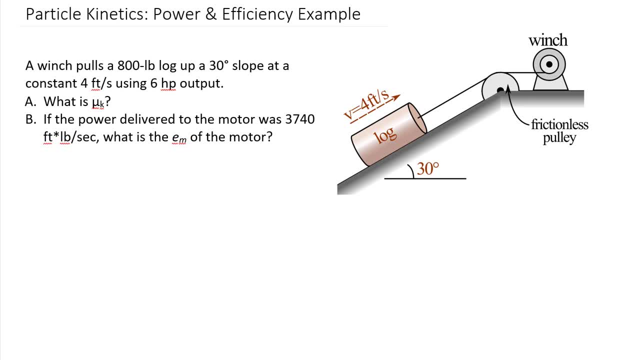 example here of a log. it's being pulled up a slope by a winch. okay, so this log has a weight of 800 pounds and we're pulling it at a constant velocity. we do need free body diagrams if you think out that we're going to some forces. we need some free. 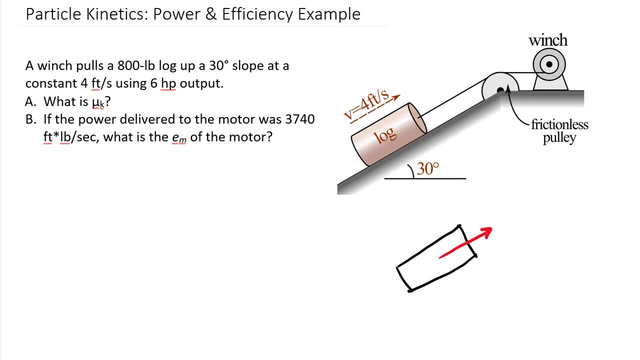 body diagrams in order to turn what those forces are. and so this is going to be the tension, the weight force, of course, pulling toward the center of the earth, we will have a normal force and also there would be a friction force. draw that along the bottom edge here. 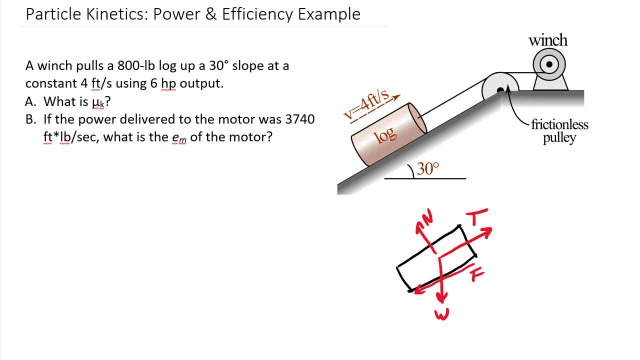 there is a force here, and there is a force here and there is a force here and there is a friction force, because we're actually going to solve for that mu sub k. okay, so we label this f sub k- is that will be a kinetic friction, pulling it up? 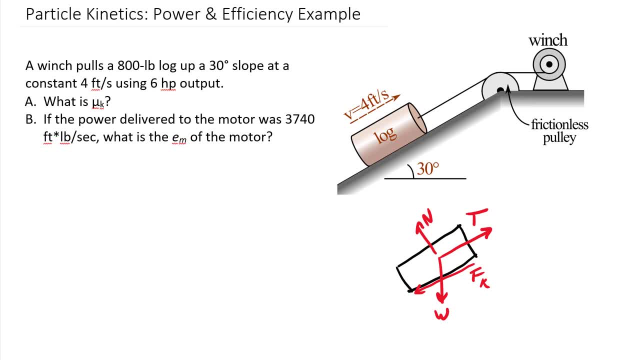 this slope, and so to think about how we would work through this problem. a couple steps here, so for part a. fundamentally we could end up computing our acceleration, which turns out in this problem because the velocity is constant. let me actually complete my free body diagram here with an axis system. 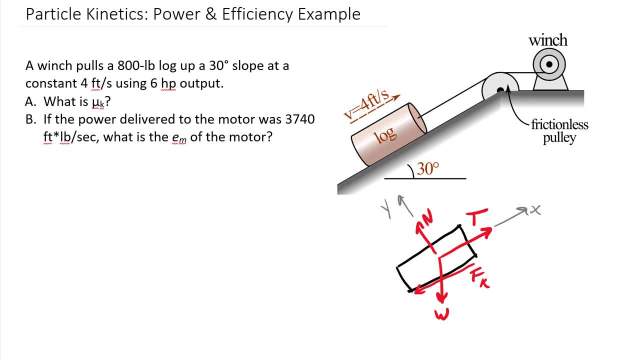 so both in the x direction and also the y direction the acceleration is equal to zero. so there really isn't a kinetic diagram. I guess we could go ahead and put the velocity here: V is equal to four as our one, and that's in feet per second. as 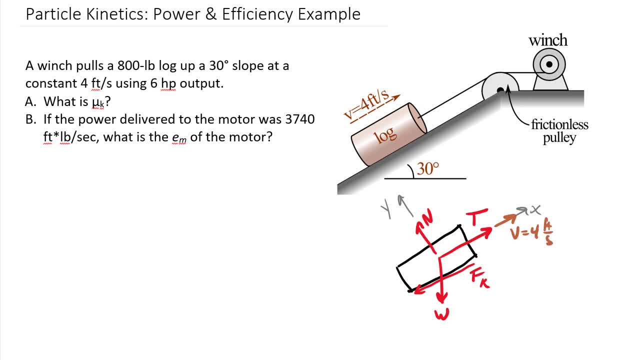 our one kinetic term, so really the. if we apply some Newtonian kinetics, it's going to look a lot like statics, right? some of forces equal zero, so let's go ahead and start there. forces going to start in the y direction is equal to mass times a sub y again here. 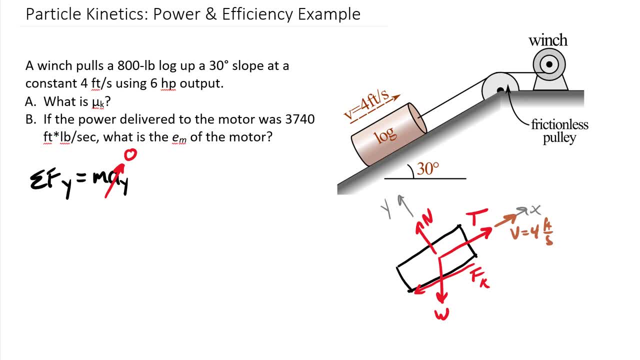 we know the a sub y is equal to zero. so on the left hand, summing those forces, we have our normal force and then we're going to have the X component of the weight. so it's going to be minus eight hundred and that's going to be the. 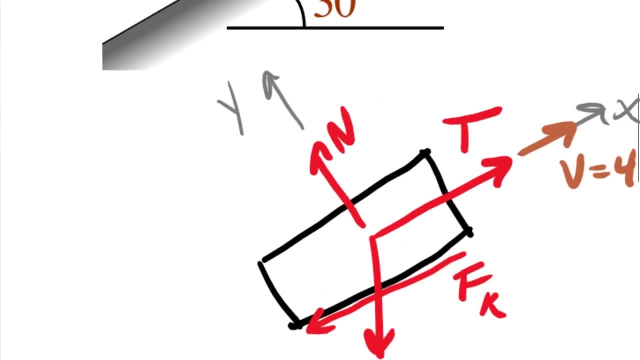 cosine of 30. again, where this is coming from is we are using a rotated coordinate system. my weight is here. if I know that this angle is 30, then also my normal force and the weight force there are going to be 30, so normal is going to. 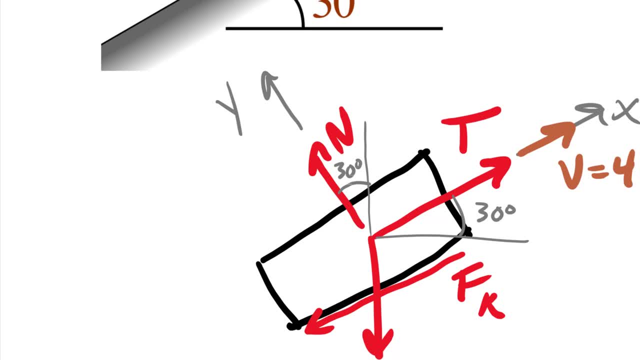 be in the y direction. the weight force is going to be 30 degrees off of the y direction. therefore, the y component is going to be cosine adjacent to that 30, so that's going to be the cosine of 30. so that's going to be the cosine of 30. 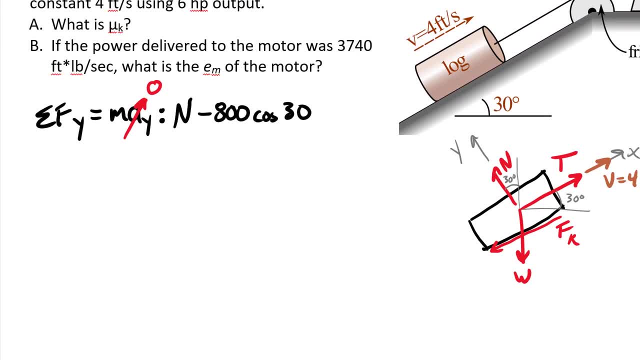 degrees. okay, so n minus 800, cosine 30, this is equal to zero. therefore we can find my normal force is equal to 692.82 pounds. do the same thing for some. our forces in the X direction. again, equal mass times a sub X. now you could have an. 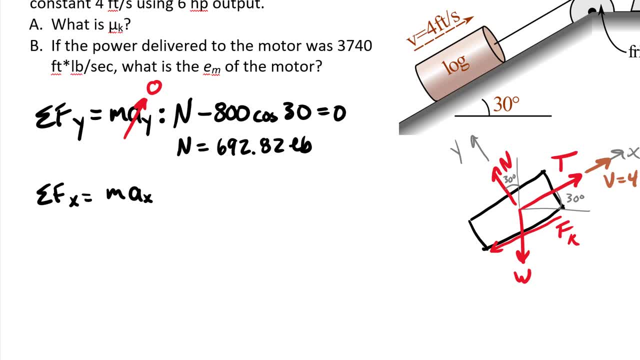 a sub X if the motor was pulling hard enough to basically be speeding this log up, overcoming that kinetic force. so that's what we're going to be doing here. kinetic friction but we have in this problem is just a balance of friction and that pulling force, so an acceleration equal to zero. so now we have the tension. 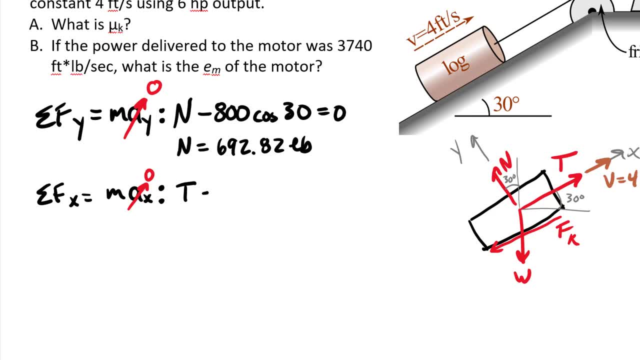 force T that's in the positive X direction, and then we're going to subtract off our friction force, that's 692.82 times our unknown mu sub K, and then additionally the weight component in that direction, so that's going to be 800, this time the sine of 30 degrees, and then we're going to subtract off our 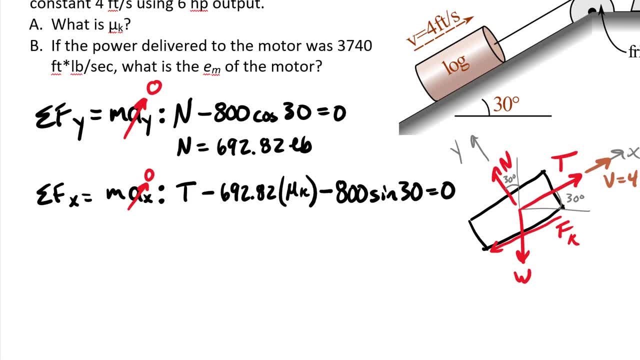 30 degrees, and that is equal to zero. okay, so we still have two unknowns. we don't know the tension. we also don't know mu sub K, so we're not out of the weeds yet, but if you think about the kind of information we have not used yet, 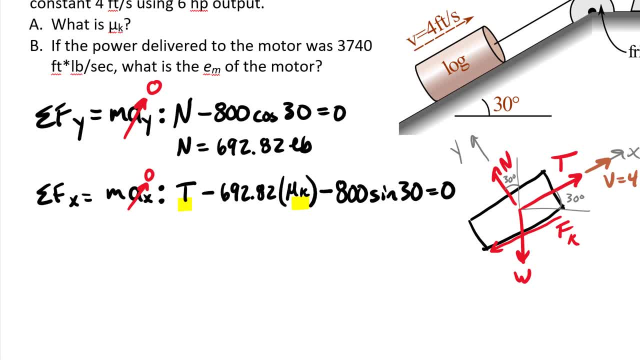 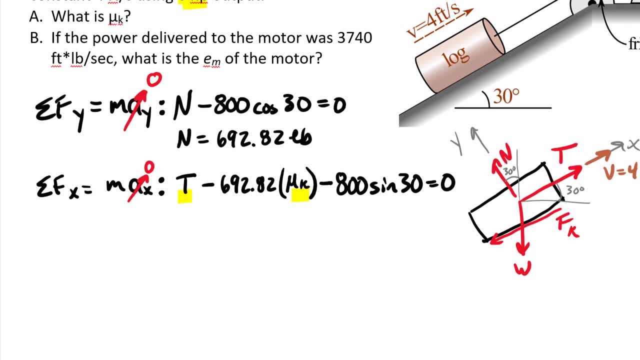 we have not used any information about our six horsepower motor. okay, so let's see if we can bring that in and solve some of that. so the other remaining unknowns. and so we are going to use power. okay, so we're going to use this power equation to find out what it's going to. 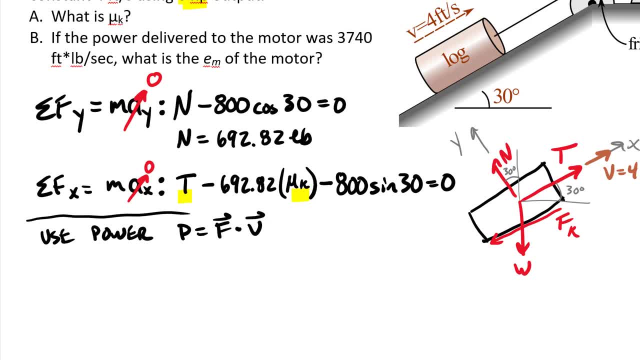 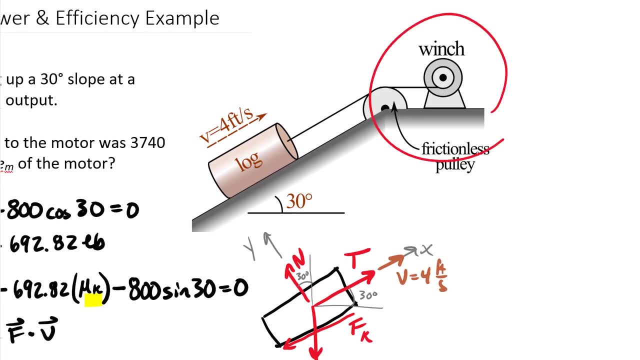 require from our input. so here are the. 56 gives me power is equal to f-dot v. okay, so we know our velocity. we know that our F, fundamentally in this problem, is our tension. okay, the reason I know that is because this power equation is basically is basically looking at, one can move per minute or may be five per minute. so 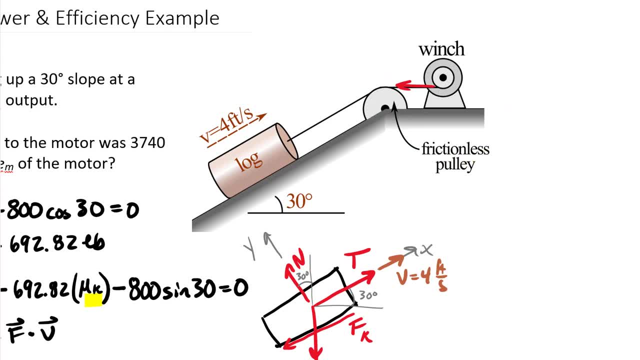 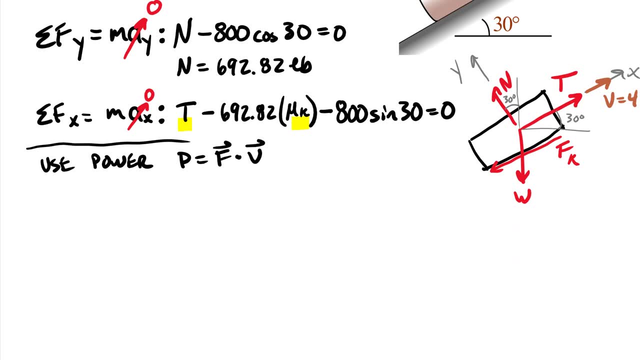 and it's pulling that tension at a given velocity. okay, so there that's how we can tell. that's basically the power as related to the winch is related to the tension. so let me write this here: there's my unknown tension and the velocity. now, because they're parallel, the dot product. 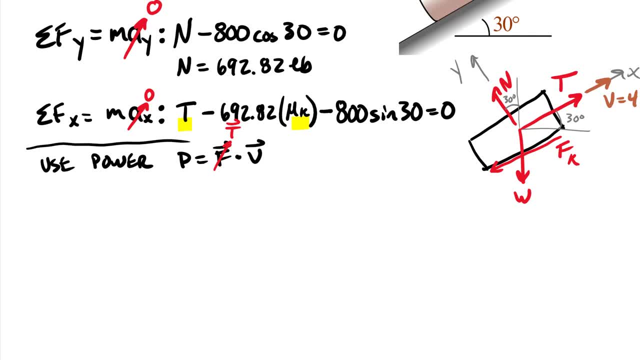 basically gives me the sum, excuse me, the product of those two. so we can write here that p is equal to times v, once again, because the tension is parallel to the velocity pulling into that rent, that winch. so we have a value for the power, we have a value for the velocity we want. 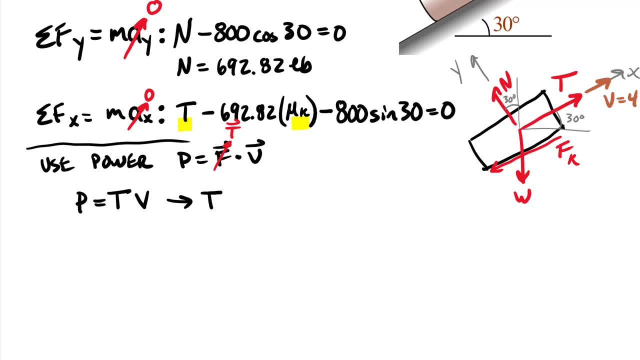 to solve for that tension. so we can rearrange this and say that t is equal to the power divided by the velocity. now the power is given six horsepower and we can convert this into feet and pounds and seconds by our conversion factor 550.. So this is in foot pounds per second. 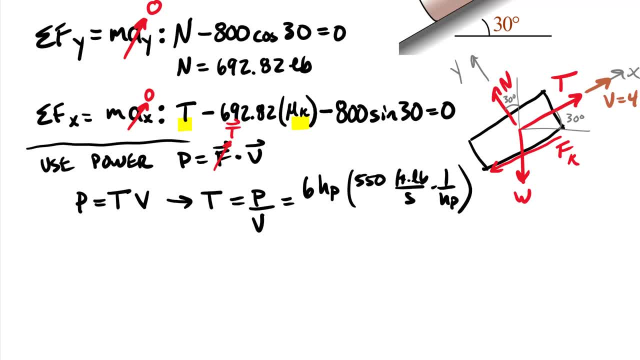 That's equal to one horsepower. Okay, so the horsepower cancels and we're left with a foot pound per second, And then we divide that by the velocity constant value of four feet per second. So that leaves us- let's see, the foot cancels. 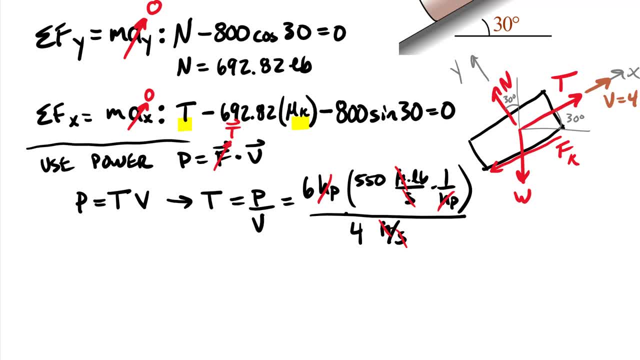 the second cancels leaves us with the pounds, which is a good unit for attention. So attention is equal to 825 pounds. We then could put that back into our equation up here. So let me call this equation one, So we'll say: into equation one. 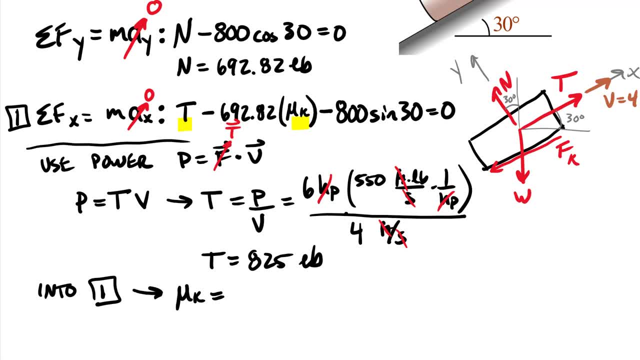 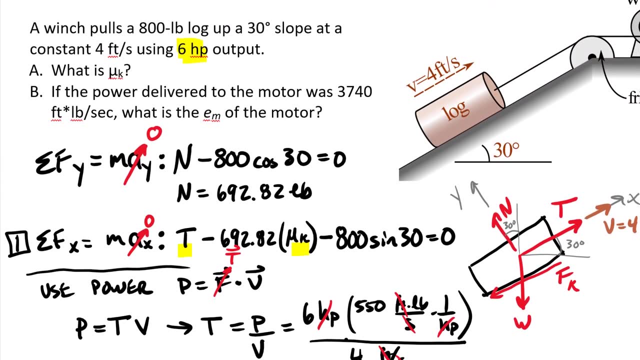 we can solve that. our mu sub k is equal to 0.613, right, And there's not gonna be any units ever on a coefficient of kinetic friction. And then in the last part of the problem, part B, it says if the power delivered to the motor 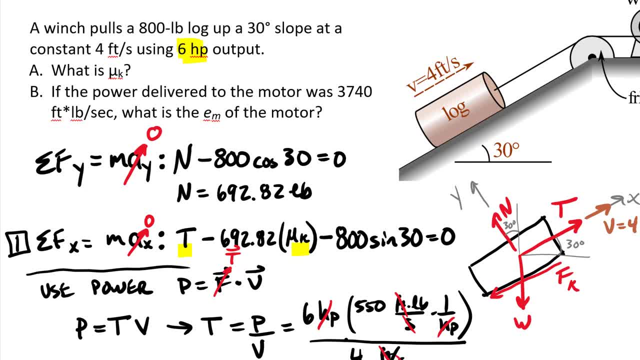 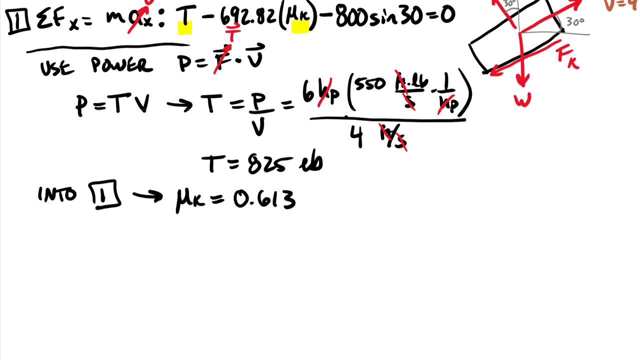 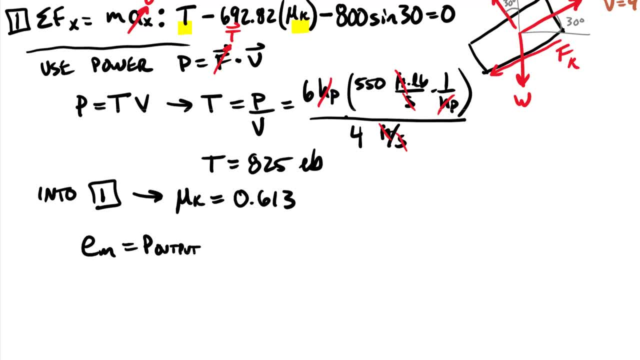 Okay, so we've got the power. Okay, so we've got the power, And that's going to be the power output divided by the power input, And so again, the output. we know we're getting six horsepower using the conversion factor. 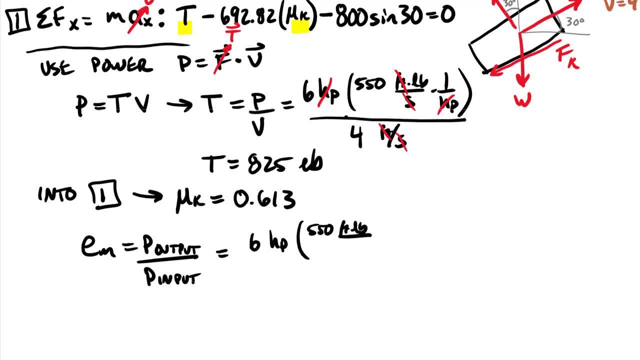 here again: 550 foot pounds per second, times one over horsepower. And then divide this by our input 3,740.. And then divide this by our input 3,740.. This is in foot pounds per second. Now all of these units are going to cancel. 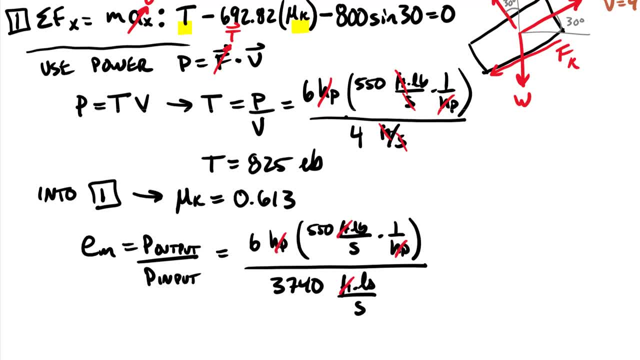 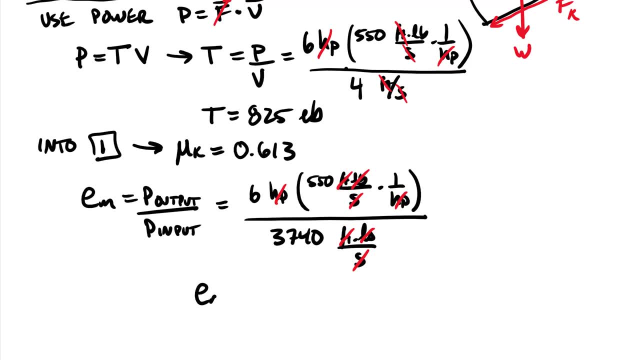 because efficiency is a unit-less ratio. Okay, so pounds, pounds, seconds, seconds. So all of those units cancel And we end up with E M equal to 0.882.. Okay, like many percentages, this comes out as a number less than one.